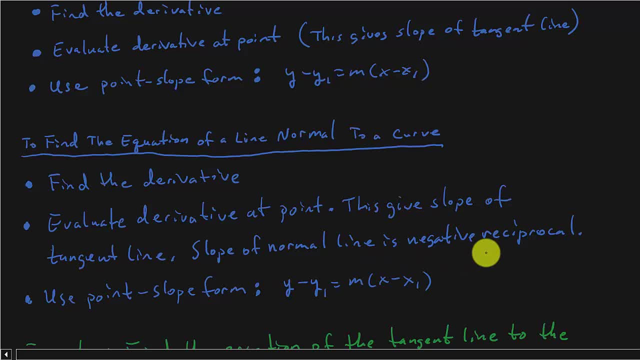 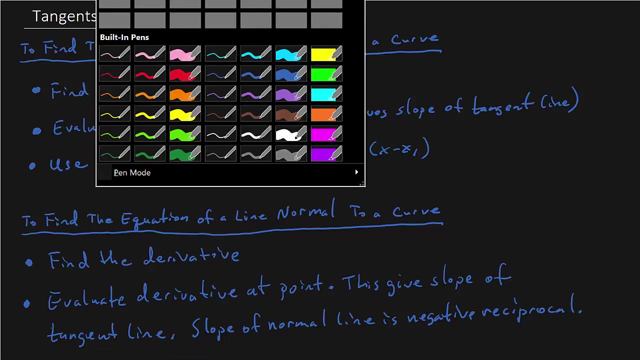 of the tangent line. Well, the slope of the normal line is the negative reciprocal of the slope of the tangent line, and then we use the point slope form. All right, so basically, what we're, what we're finding here is: um, let me show you. so let's just say you have a graph here. 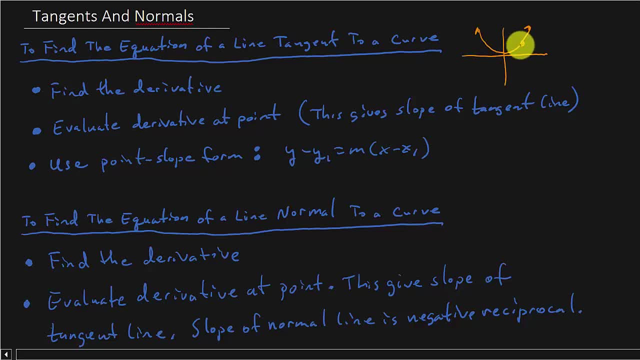 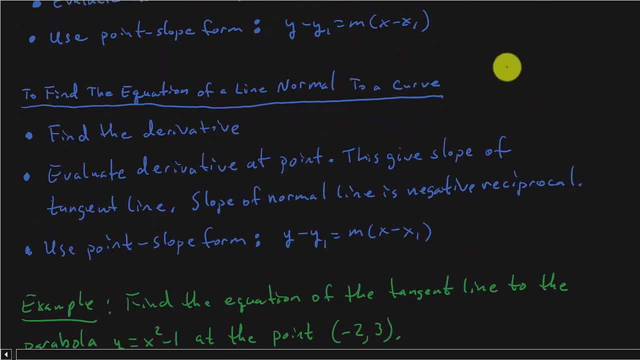 we'll just draw a parabola and you have a point here. that's the line that's tangent to that curve at this particular point right here. This is your tangent line and that's the equation of the line that we're trying to find. Now for the normal line. well, let's just go up here. 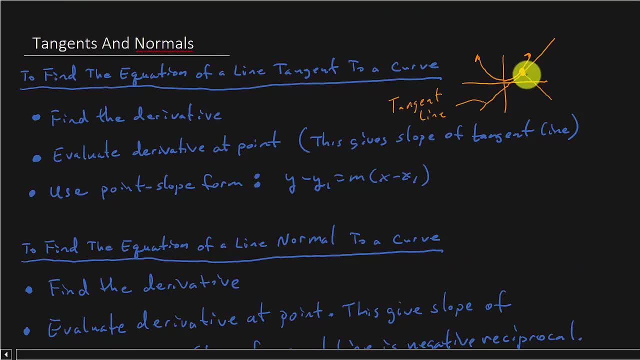 the normal line. you have a line that is perpendicular to the tangent line. at that point, This is your normal line, right here, All right, and you see that the. so you have the tangent line and the normal line. they're perpendicular. Well, what do we know about perpendicular? 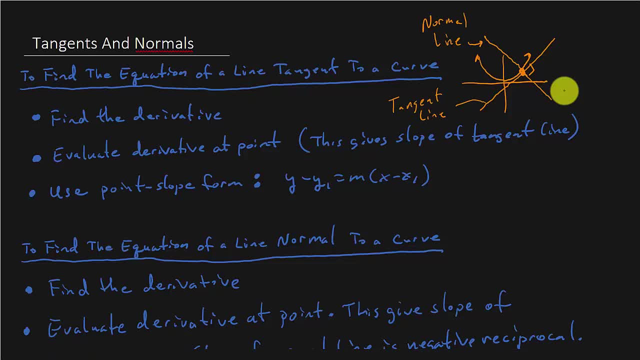 Well, if you look at this graph here, we have two perpendicular lines. They're slopes or negative reciprocals of each other. Okay, and that's why, when you're looking for the equation of the tangent line, well, you evaluate the derivative that gives the slope. 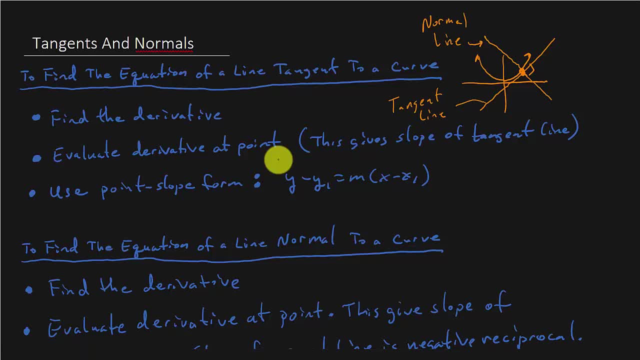 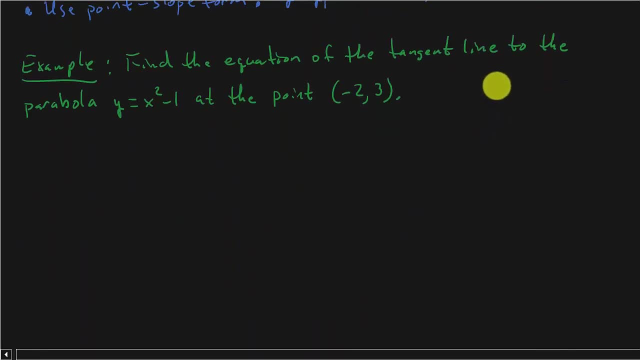 of the tangent line, and so the slope of the normal line would be the negative reciprocal of that. All right, all right, so let's, let's get started on some examples. We've got, I think, four examples to work: two for the tangent line, two for the normal. 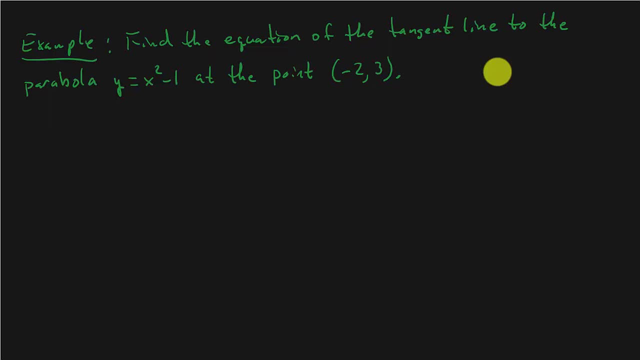 line, and then we have a word problem. So hang around for the whole video. you'll learn some stuff, Alright. so find the equation of the tangent line to the parabola: y equals x squared minus one at the point negative two, three. 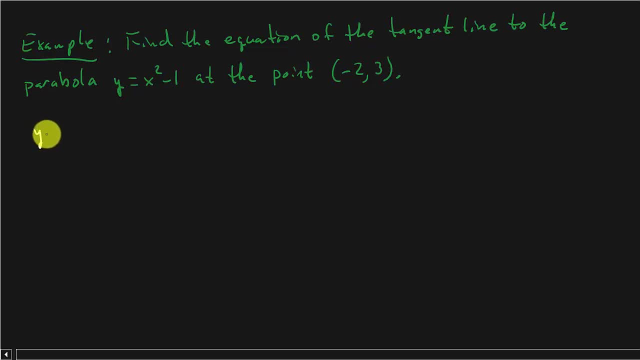 Alright. so what does it say? Let's write the problem down. So it says: find the derivative. alright. well, what's the derivative? Y prime is two, x. okay, there's the derivative of x squared minus one. And then we evaluate the derivative at the point. 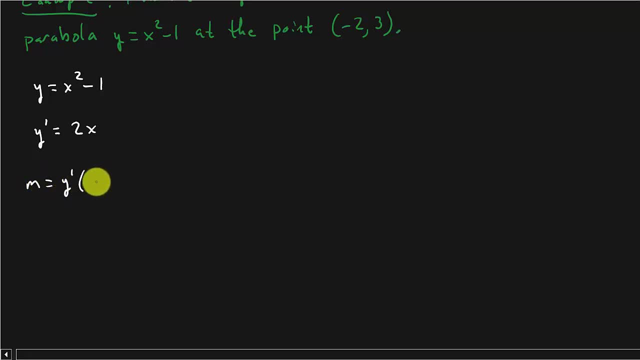 So the slope is y prime of now. I'm evaluating it at the point. but notice see, I only have an x variable. Well, so all I need is the x coordinate. I just need to plug in the negative two, And so that's going to be two times negative two, which is negative four. 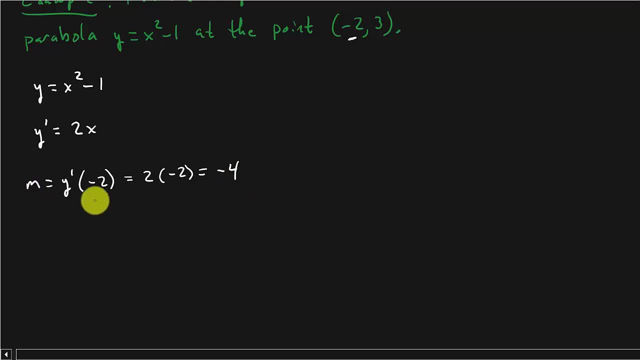 That's the slope of the tangent line. okay, And then we use y minus y one equals m times x minus x one and we plug everything in. So look at this, You know I'm trying to erase that white line. that wasn't letting me. 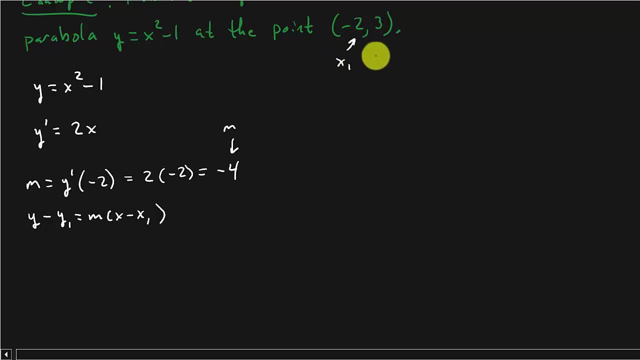 So we know that's m, this is your x one and this is your y one. So we plug them in. So y minus three equals negative four times x, and then minus a negative two is going to be plus two, And then go ahead and solve it for y. 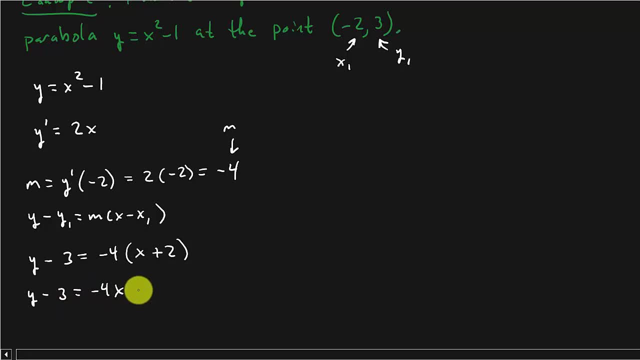 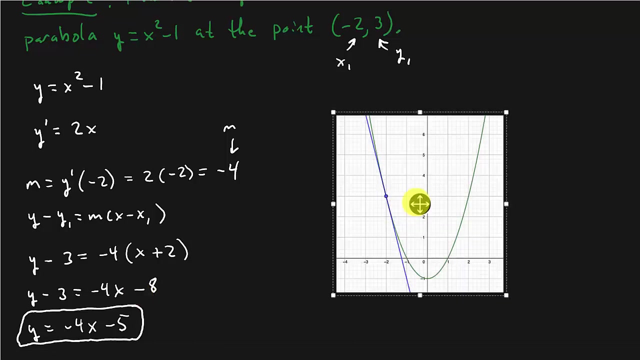 So y minus three equals negative four x minus eight. Okay, So y equals negative four x minus five, And there's the equation of the tangent line. All right, So now let's just let's see what we found. Okay, So I've graphed them. 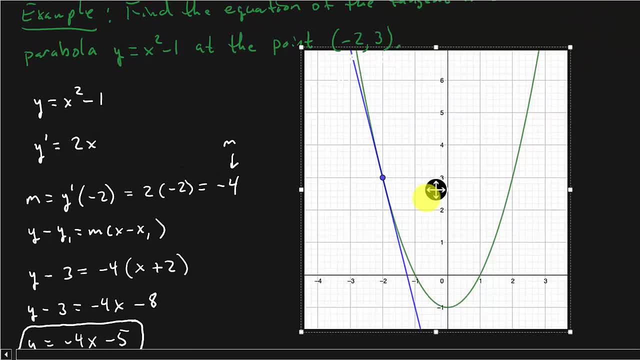 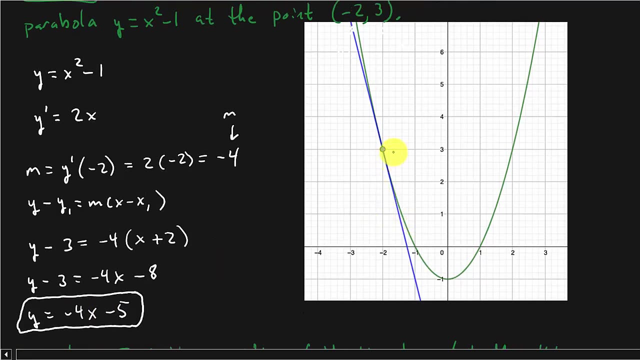 All right. So that's what it looks like. The green, that's the graph X squared minus one, Okay, And then the blue line, that's your tangent line, That's the line Y, equals negative four x minus five. 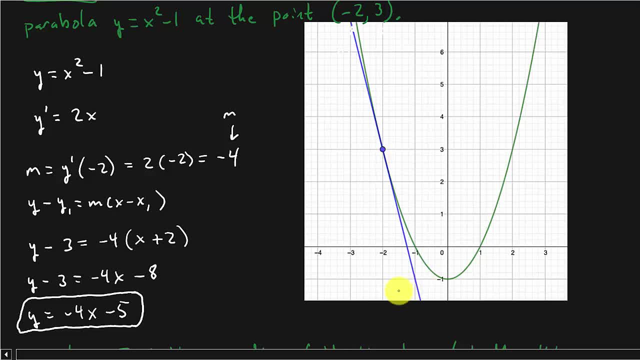 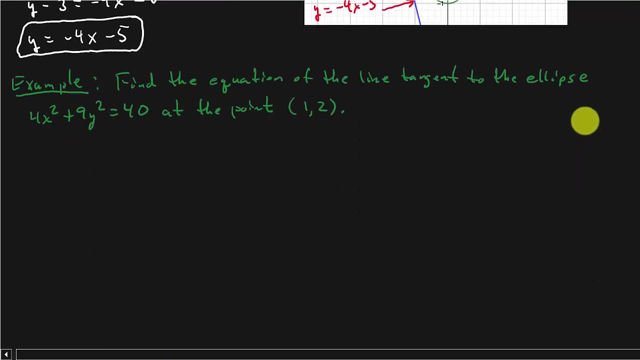 And this is your point: negative two, three, And that's what we found. The equation of this, the equation of this blue line right here: Y equals negative four, x minus five. All right, All right, Let's look at the next example. 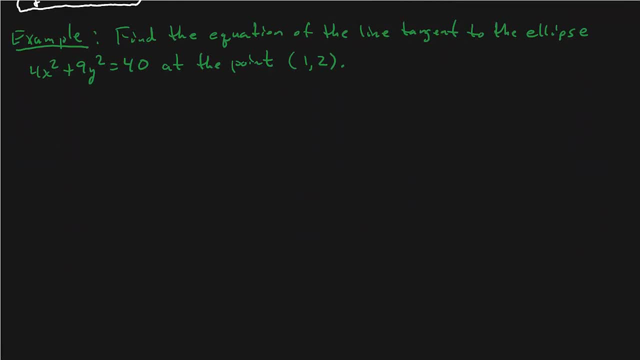 Okay, Okay, All right. So find the equation of the line tangent to the ellipse: four x squared plus nine y squared equals 40 at the point one. two. All right. So four x squared plus nine y squared equals 40.. So we have to find the derivative. 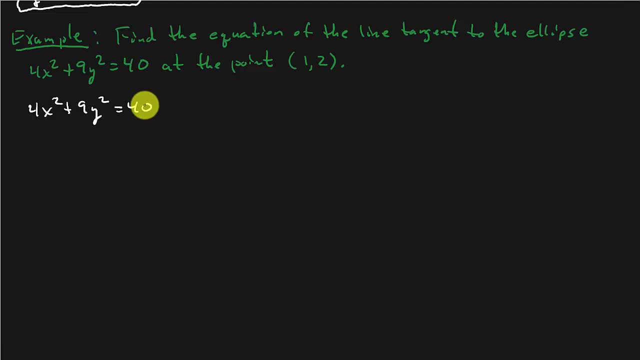 Okay, All right, We should remember how to do this implicit differentiation. So that's eight x plus 18 y times y prime equals zero, All right. And then we solve for y prime. So 18 y y prime equals negative eight x. 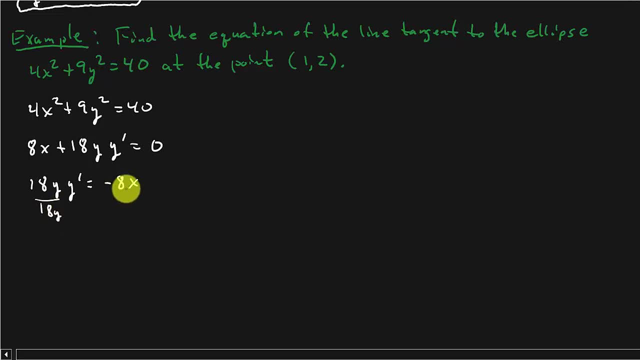 Divide everything by 18 y, And so we get y. prime is equal to negative. four x over nine y. All right, So there's your derivative. So now, what do we do? Well, we evaluate the derivative at the point. Now, this time, notice how we have an x and a y. 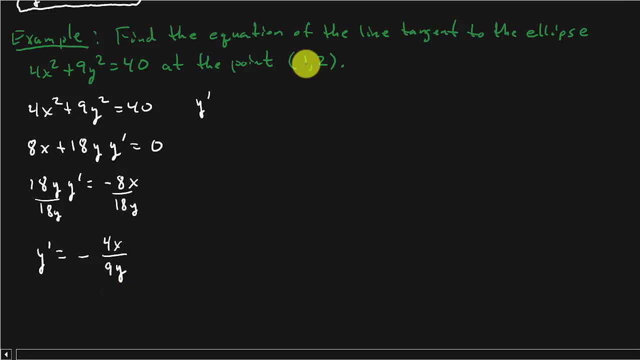 Okay, So we've got to plug the one in. Okay, We plug the one in for x, the two in for y, And so that's going to be y prime of one, two, And that is going to be negative four times one over nine times two. 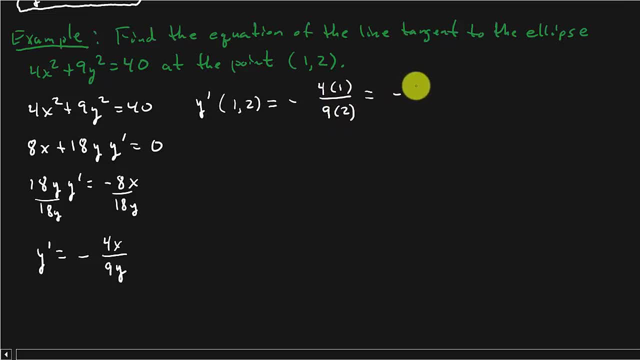 All right, And so that's going to be negative two over nine. And let me go ahead and note this is m equals. That's your slope: Negative two. Negative two nines. All right, Now we use: y minus y one equals m times x minus x one. 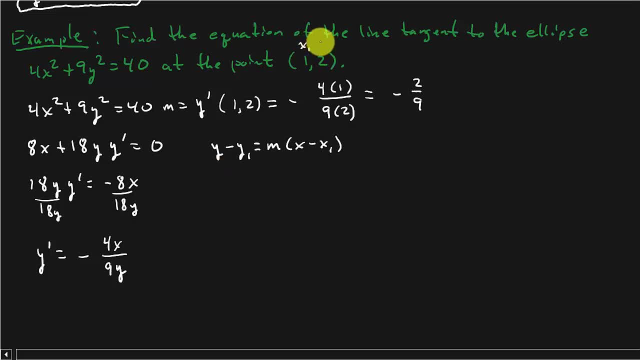 So we've got remember: this is x one, this is y one, and that's m your slope. And so y minus two equals negative two nines times x minus one. Y minus two. Y minus two: equals negative two nines. x plus two nines. 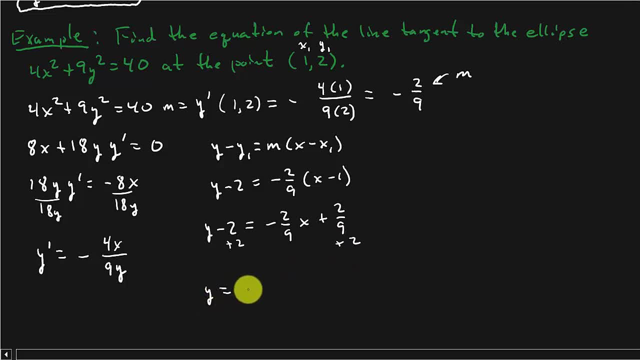 And so now I'm going to add two to both sides. So y equals negative two, nines x plus what is that? is that 20 over nine? And so there's the equation of your line. All right, Now let's see what this looks like. 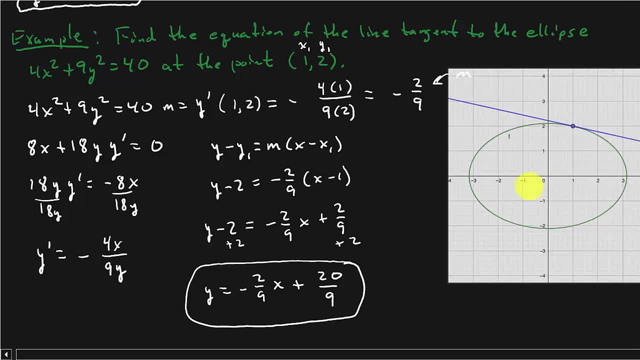 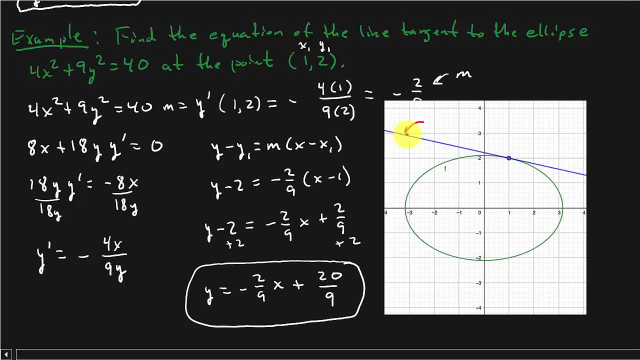 Okay, And there's what that graph looks like And here's your tangent line: Y equals negative two nines x plus 20 over nine, And this is the equation of your ellipse: Four x squared plus nine, y squared equals 40.. 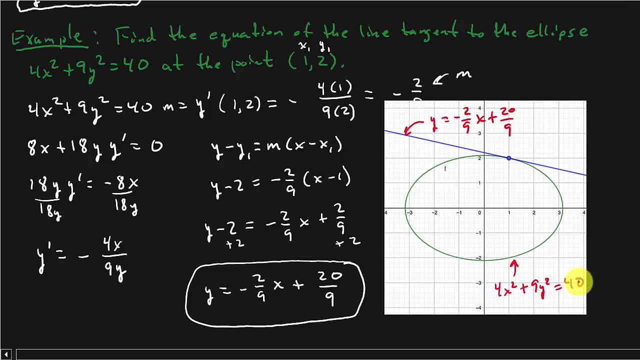 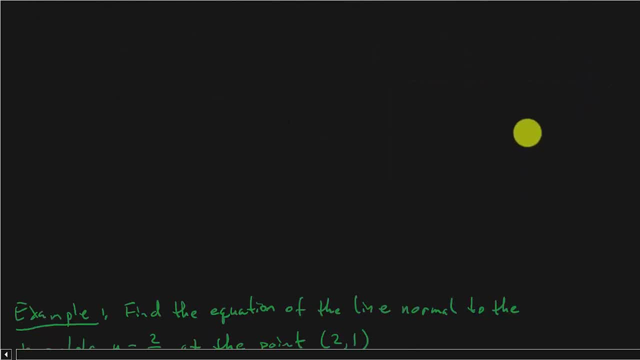 All right, All right, so let's move on to the next one. So that's, that's finding the equation of the tangent line. All right, So now let's look at some problems where we find the equation of the normal line. 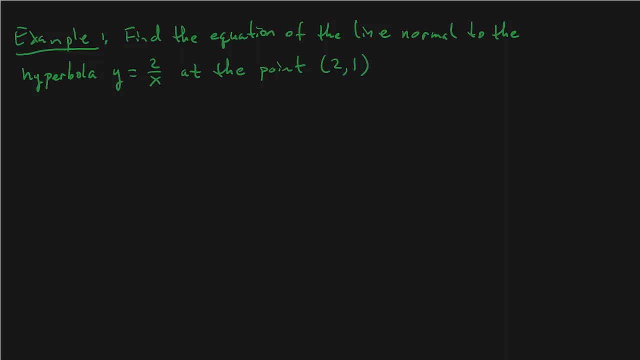 So it says: find the equation of the line normal to the hyperbola: Y equals two x At the point, At the point two, one. All right, So let's find the derivative. So we've got y equals two over x. 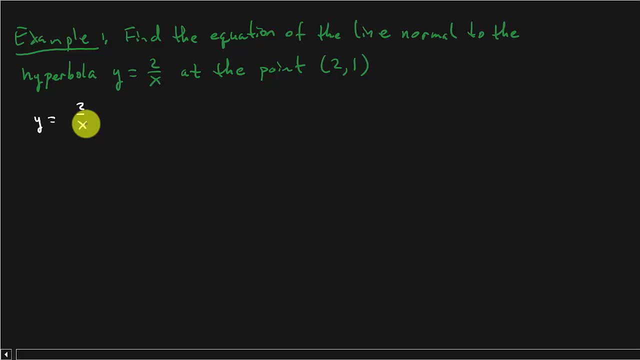 All right, Now let's let's go ahead and find this derivative, And one thing that I would, I would recommend you do, is: y equals some number over x, It. it seems like this: this comes up. well, you know, not all the time, but it comes up. 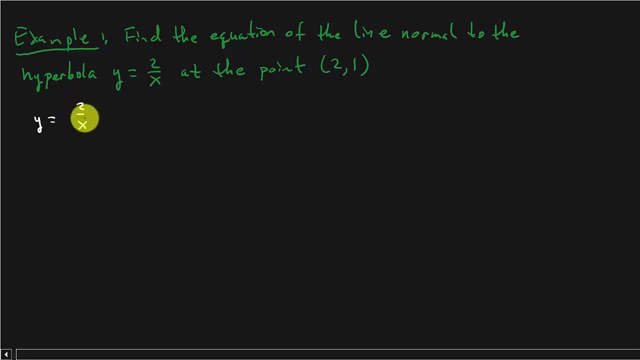 quite a bit in calculus where you have a number over x And you know you can take this derivative by rewriting it as two times x to the negative one and using the power rule. So y prime would be negative two x to the negative two. 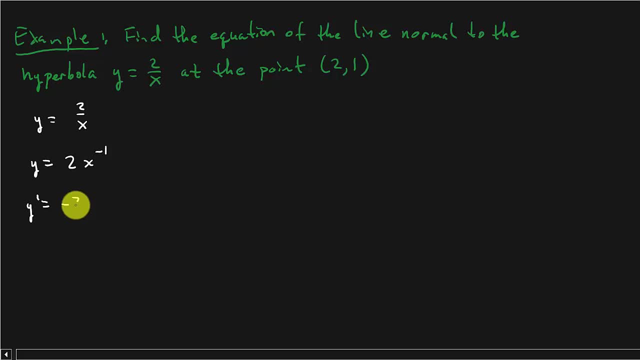 x to the negative two And y prime would be y prime, Y prime, y prime. So y prime is negative 2 over x squared. So what I've done is I just when I see a number over x, I just know it's negative that number over x squared. 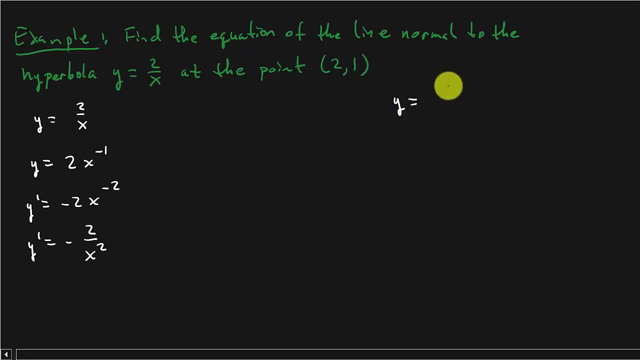 So see if you have- let's say you have- y equals c over x, some constant over x Over x. So you get y equals c times x to the negative 1. So y prime is negative, c, x to the negative 2.. 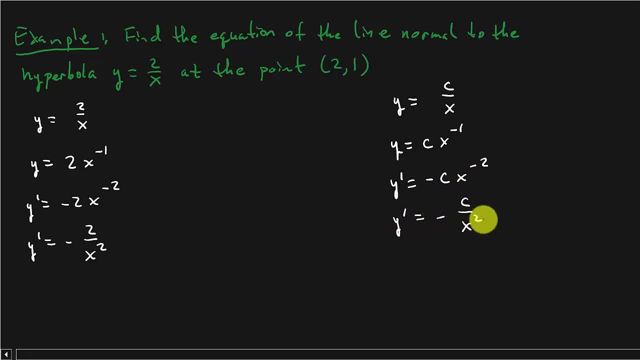 So y prime is negative, c over x squared. What I've done is I've just memorized it. So if you have a constant over x to the first power, just memorize it's negative that constant over x squared. Okay, It'll save you from having to rewrite it like this: do this step and then rewrite it with the exponent positive. 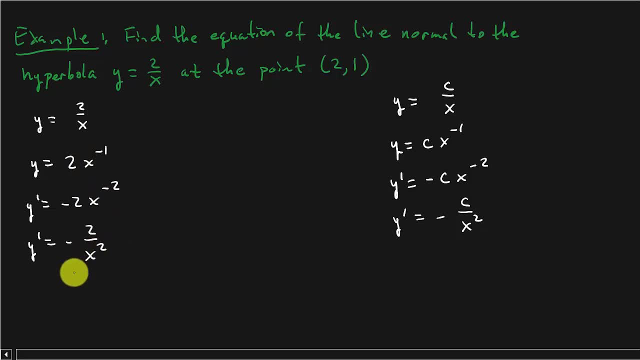 Okay, If you want to do that, that's fine. If not, that's fine. Okay, Your teacher may not want you to memorize it. Your teacher may want you to write all this out. If you're in my class, just you can go from here to here, That's fine. 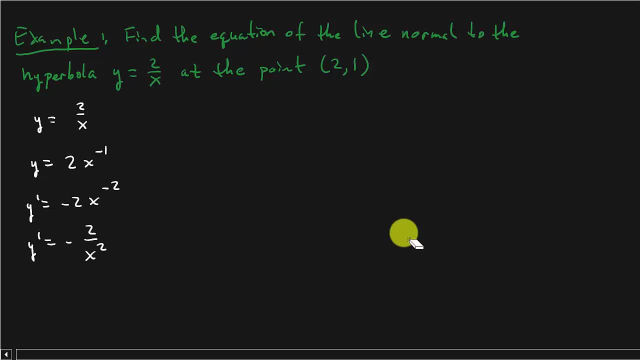 And you know, as often as it comes up, You know you'll probably end up memorizing it anyway. All right, So let's do y prime of okay. so we've got to evaluate the derivative at that point. 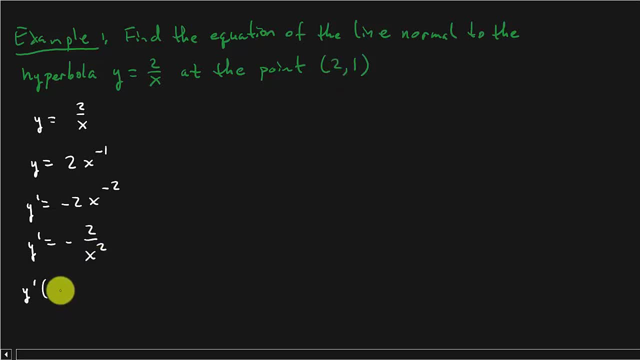 So I just need to plug the 2 in, because all I have is an x value. So that's y of 2 is equal to negative 2 over 2 squared, which is negative 1 half. All right, So. 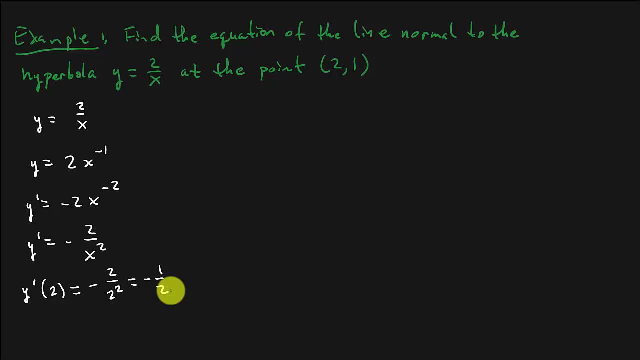 So we get: y prime of 2 is negative 1 half. That's not the slope of our line, is it? No, Because they're wanting us to find the line normal to the curve. So that means our slope is the negative reciprocal of this. 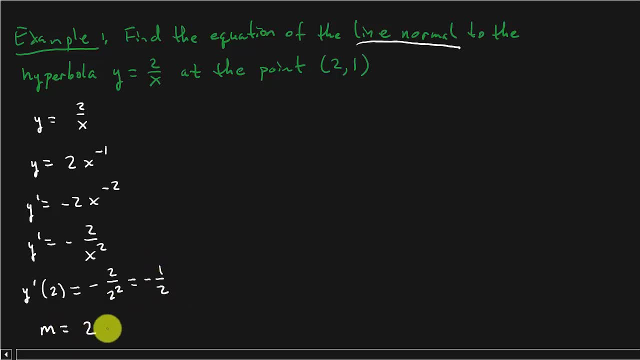 So what's the negative reciprocal? Well, you flip it and change the sign. All right. So there's your slope, There's m, there's x1, there's y1.. So y minus y1 equals m times x minus x1.. 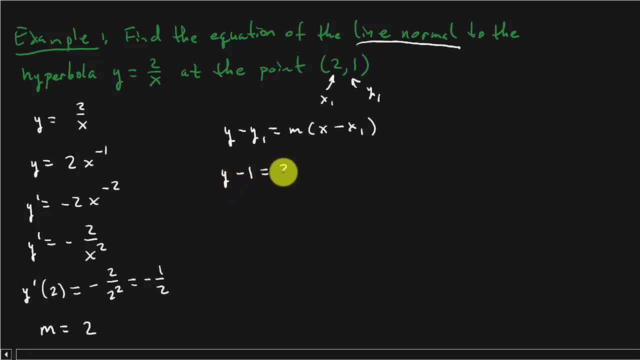 So plug it in: y minus 1 equals 2 times x minus 2.. So y minus 1 equals 2x minus 4. Y equals 2x minus 3. And there is the equation. Okay, So we've got it. 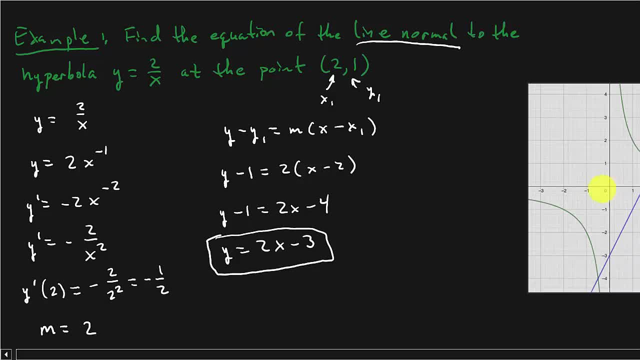 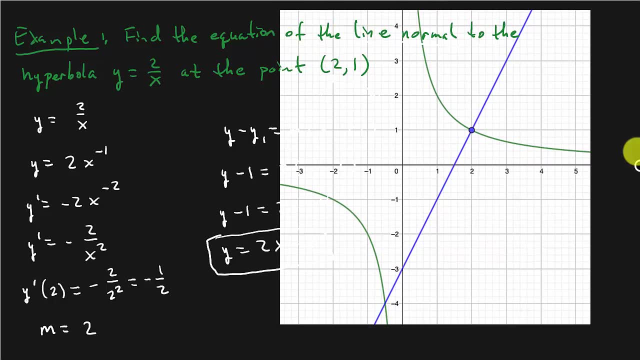 The're the positionPUi plus 1 plus two. That's the line, of your line. And once again, How about we look at the picture of it? See, Make it a little bigger. And there it is. And see, look. 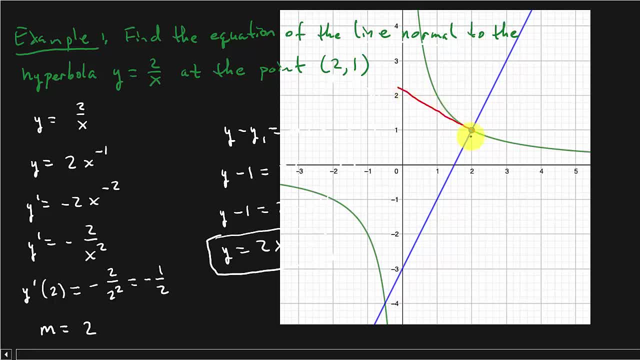 If you drew in, see, you can draw in the tangent line right here. See, if we kind of sketch that in, There's your tangent line, The blue line is your normal line. This right here is the graph. y equals what was it? 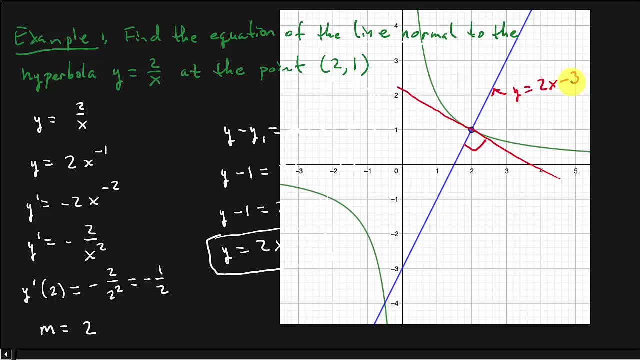 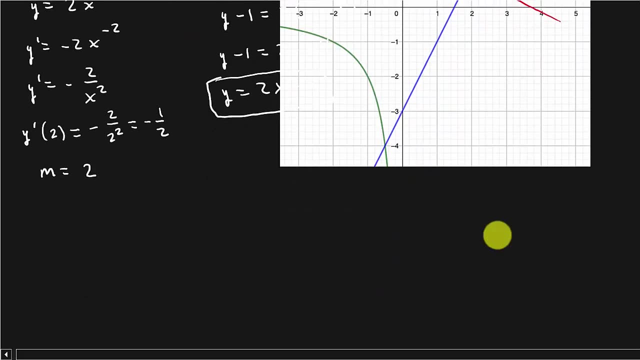 2x minus 3.. Yeah, and then the green line is your: y equals 2 over x. but yeah, this is this blue line. that's your normal line, and see it's perpendicular to the tangent line right here. all right, all right, let's. 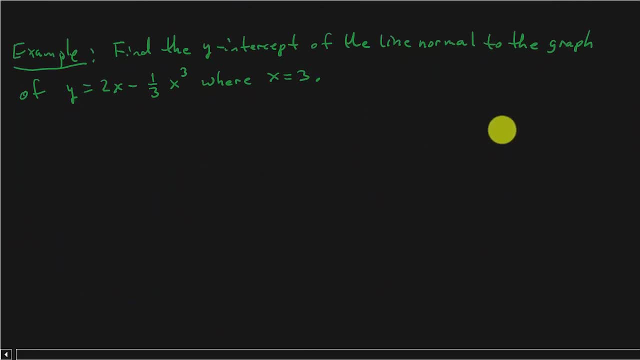 look at another one. we got this one and then we have a word problem to do and- and i hope you're still well, i mean, if you're watching the video, you are, but watch this problem. okay, don't get bored and just click the video off, because look at this, they only give us x equal 3. you see that? 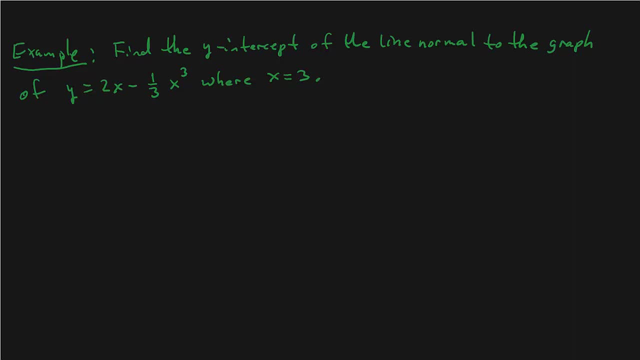 all right. so find the y intercept of the line. normal to the graph of y equals 2x minus one third x cubed where x equals 3. so they're not asking us to find the normal line, they're asking us to find the y intercept of the normal line. but to do that we have 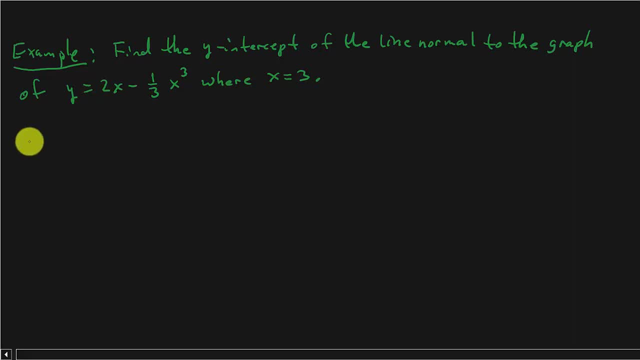 to find the y intercept of the normal line. and we have to find the y intercept of the normal line to find the equation of the normal line. and so we have: y equals 2x minus one third x cubed. there's our curve. now find the normal line to this graph. now, what has it been telling us in the other? 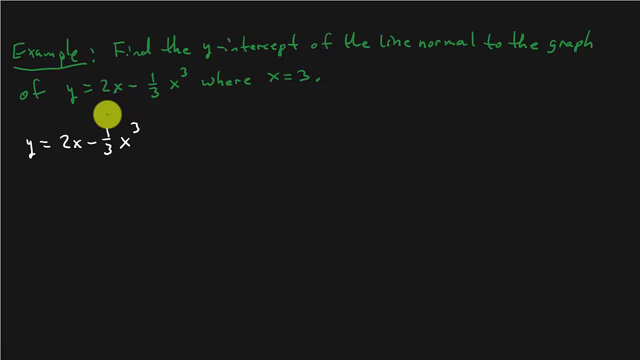 problems. in the other problems it's been saying: find the line normal to the graph or tangent to the graph. at this point they don't say: at this point they say: where x equals 3. well, in order to find the equation of a line, we've got to have a point on the line, don't we? we need to know the. 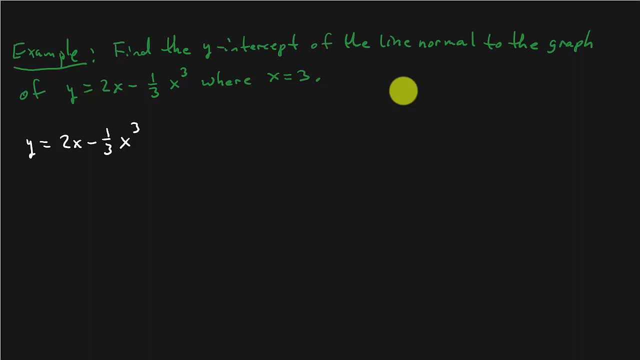 slope and we need to know a point on the line. well, they tell us that x equals 3. so if x equals 3, so i've got the x coordinate of my point. so what's the y coordinate? well, how do we find the y coordinate? well, you take this and you just 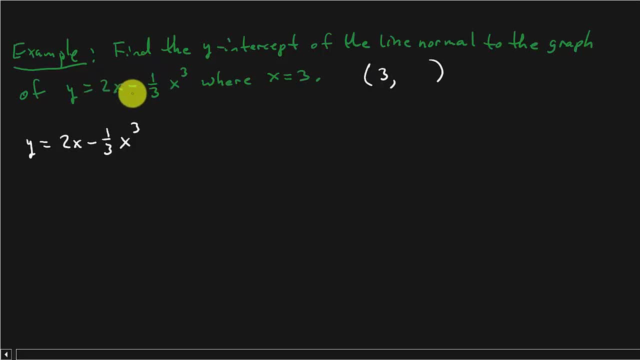 plug it back in to the original function to get your y right. if x is 3, we plug it in here for x and that'll give us y, and so i've got y equals. let's do this. y of 3 is equal to 2 times 3 minus. 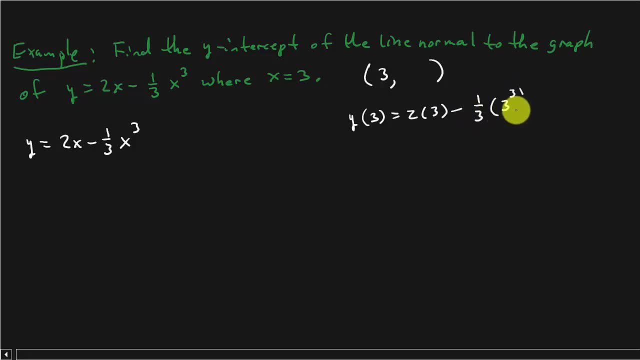 one third times 3 cubed. so that's going to be 6 minus 9, which is negative 3. so now look, you can read the problem. now find the y intercept of the line normal to the graph of y equals 2x minus one third x cubed at the. 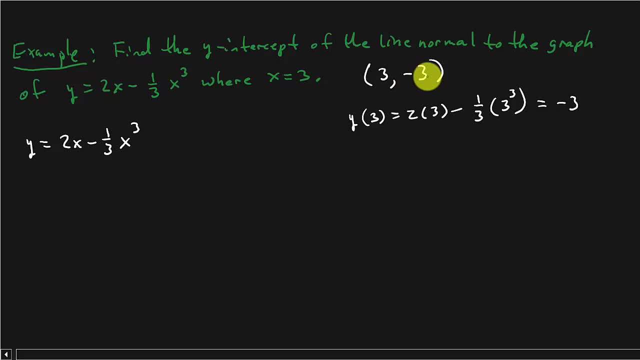 point 3 negative 3. so sometimes they may just give you the x coordinate. well, if they do, just plug it back into the, into the function to get your y coordinate alright. so let's take the derivative. so y prime is 2 minus x squared and so y. 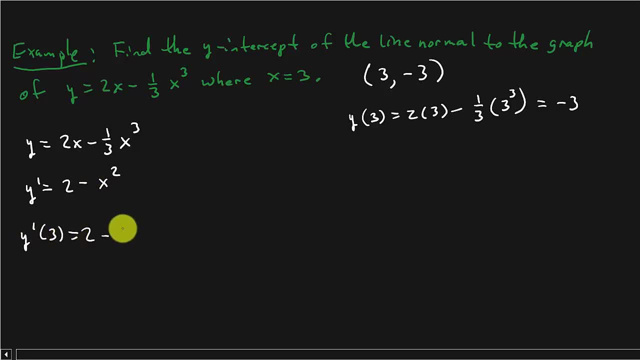 prime of 3 is 2 minus 3 squared. what is that? negative? negative 7. okay, so the slope is what 1- 7th. so the slope is what 1- 7th, because we're finding the normal one. so the slope is the negative. 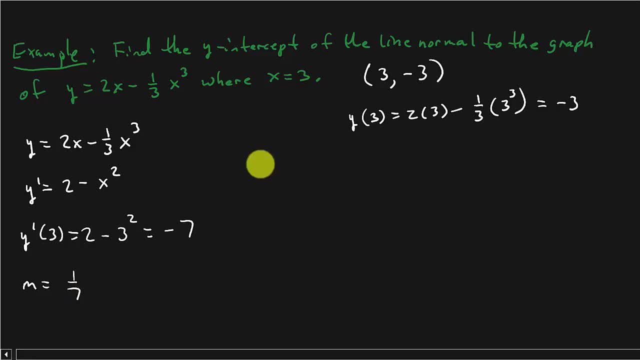 reciprocal. alright. so I've got y minus y 1 equals m times outside, minus x1, and so y minus negative 3 is plus 3, equals 1 7th times x minus 3, help out. so y plus 3 equals 1, 7th x. 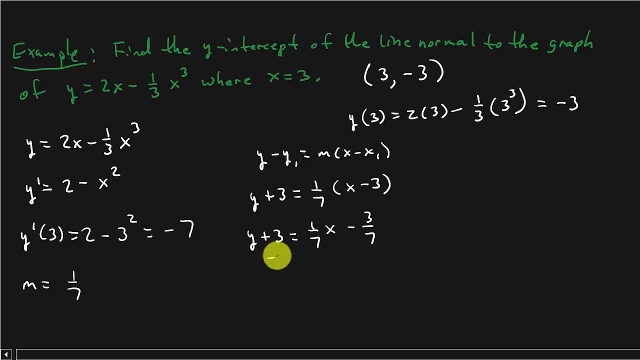 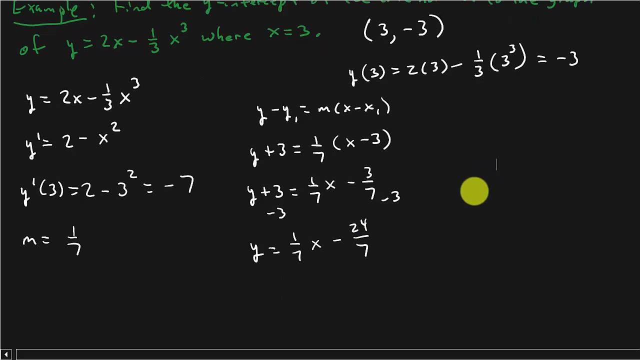 minus 3 sevenths. and then I'm going to subtract 3, so y equals 1 seventh, X minus, and that's going to be 24 over 7. and and what? what were they wanting us to find? they were wanting us to find the y-intercept. so the y-intercept is the. 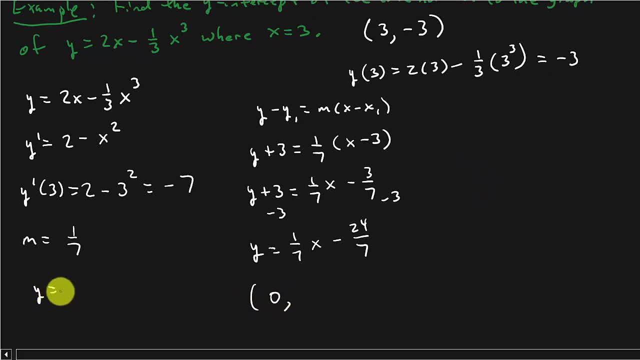 point zero. remember, if you have, y equals mx plus B, M is your slope and the y-intercept is the point 0, B, whatever that constant is. so that's 0 negative 24 over 7. so that's what they were wanting us to find, but we did have to find the 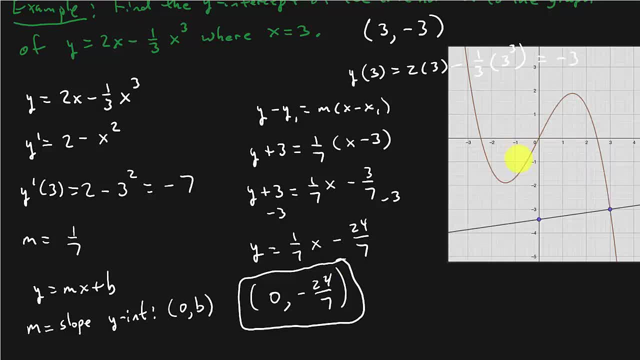 equation of the normal line, and so let's see what that looks like. you can see that the y-intercept is the point zero, so that's what they were wanting us to find. but we did have to find the equation of the normal line, and so let's see what that looks like. 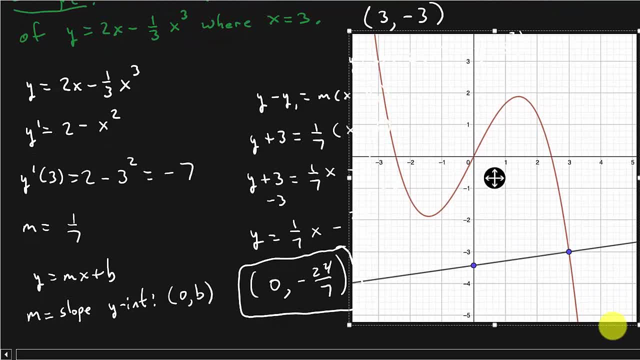 so that's this right here. and so here's your curve. y equals 2x minus 1 third X cubed. here's your line. that's normal to that point. okay, see, if we wanted to, we could you know if we, if we. that's not a very good drawing, but there's your. 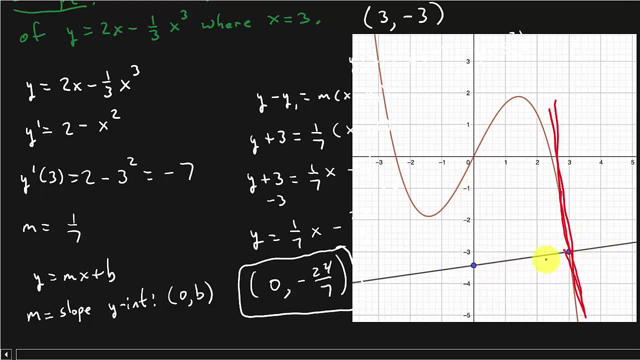 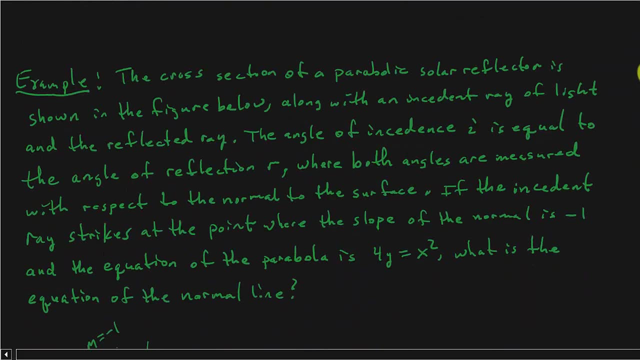 tangent line, and you know that doesn't look good at all. here's your normal line. it's perpendicular to the tangent line and that's what we found right there. we found the y-intercept, all right. so we've got our last problem. this is a word. 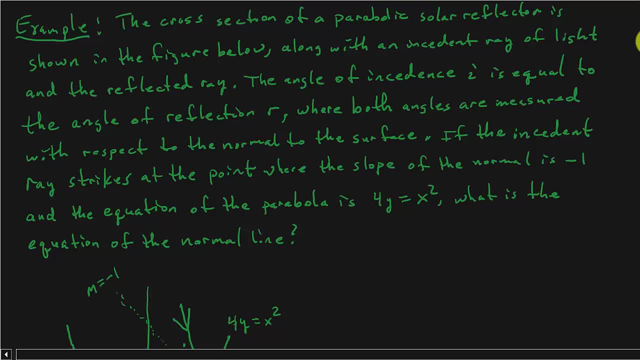 problem. so let's look. the cross-section of a parabolic solar reflector is shown in the figure below, along with an incident ray of light and the reflected light. the angle of incidence I is equal to the angle of reflection R, where both angles are measured with. 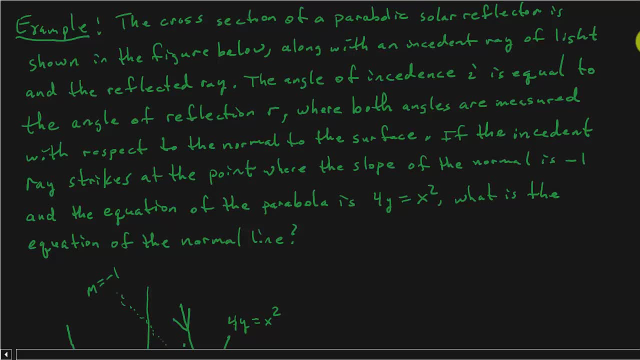 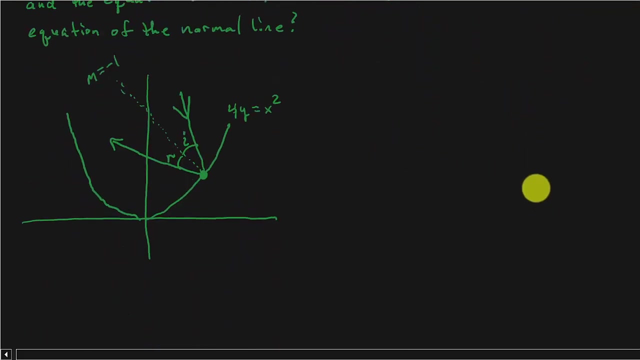 respect to the normal, to the surface. if the incident ray strikes at the point where the slope of the normal is negative 1 and the equation of the parabola is 4y equals x squared, what is the equation of the normal line? okay, so that's a lot there, but let's, let's see what we have to find. so we have our we. 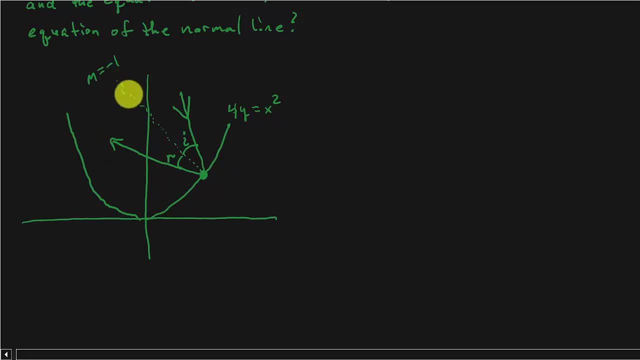 have our parabola right here. we have the normal line right here. it's that dotted green line. let's just kind of put that in red. that's your normal line, okay, and the slope of this normal line is negative 1. well, they want us to find the 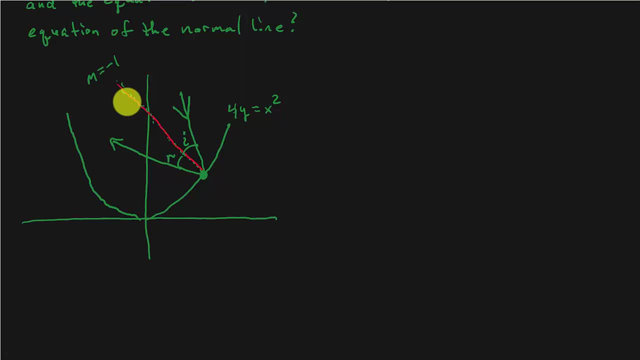 equation. okay, they want us to find the equation of the normal line, so we're going to do it. what do we need? well, we got the slope, but look, we need the coordinates of that point, don't we? and basically, what's happened here? see lights coming in and 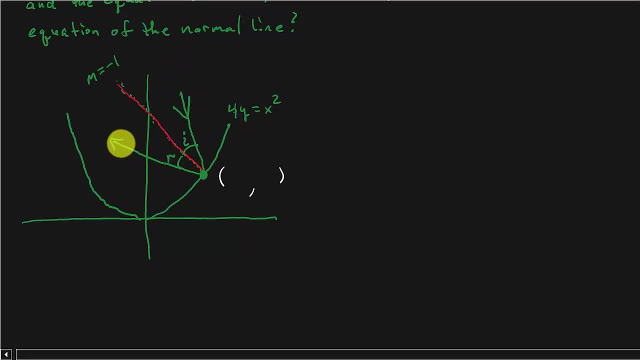 it's reflecting off. okay, alright, so. so how in the world are we gonna find the Slope, or the equation, this line? well, how are we going to find those point coordinates? Well, let's look at this. Slope of normal line is equal to negative 1.. 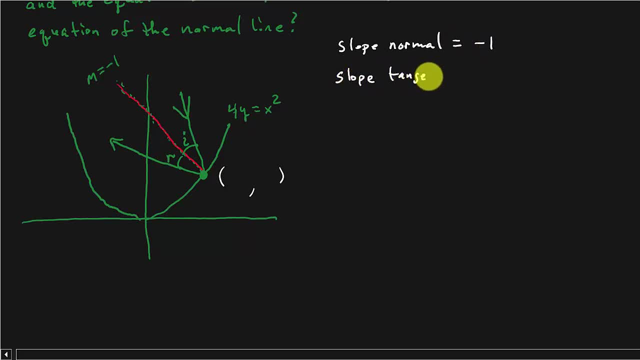 So that tells us the slope of the tangent line is the negative reciprocal of that. So I flip it and change the sign So this is negative 1 over 1, so that would be 1 over negative 1, but change the sign so that would be a positive. so the slope of the tangent line is 1.. 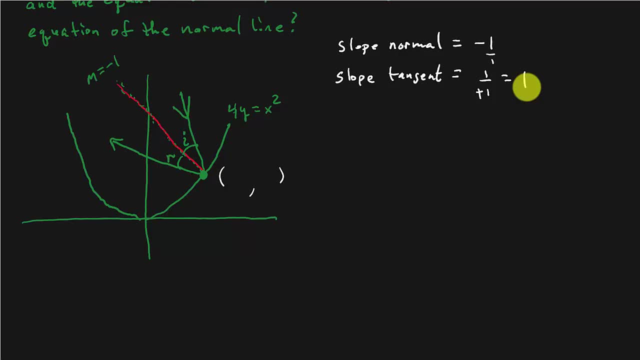 All right. So how does that help us? Well, look at this: 4y equals x squared. So if I take the derivative of this, let's take the derivative. That's 4y. prime Implicit differentiation Derivative of 4y is 4 times y, prime equals 2x. 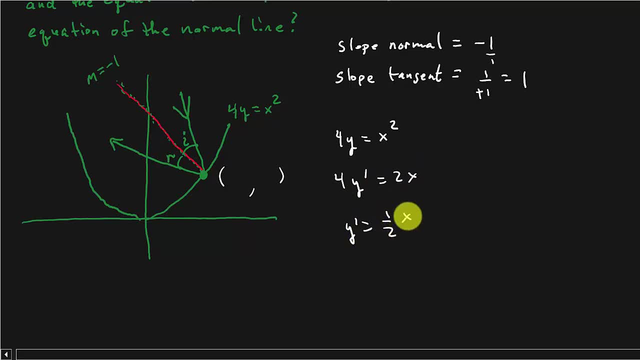 So y prime is 1 half x. You can see that. So what this means is I'm plugging some number in for x and getting 1 as an answer. Right, That's the slope of the tangent line. So I need to know if 1 half is equal. 1 half x is equal to 1, 1 half x is equal to my slope. 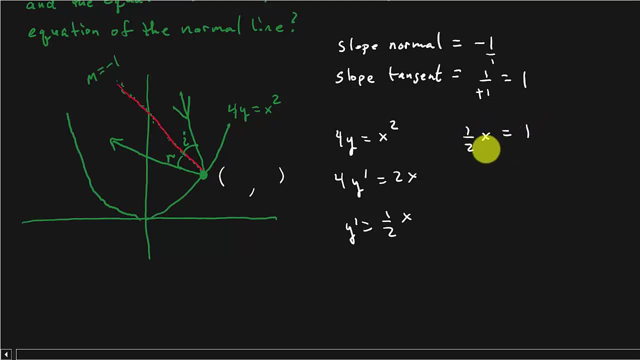 What x value is that? Well, I mean, obviously that's 2.. We can see that. So x equals. see, if I multiply everything by 2, I get x equal to 2.. So look at that, That's the x coordinate. 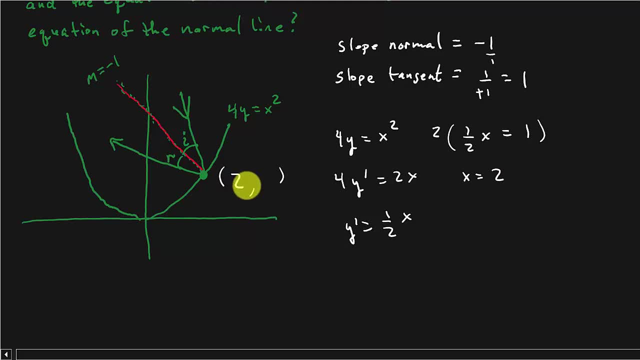 You see that That's the x coordinate of that point. Well, what do I need now? Now I need the y coordinate. So if I take 4y equals x squared and I replace the x with 2, that's 4y equals 2 squared. 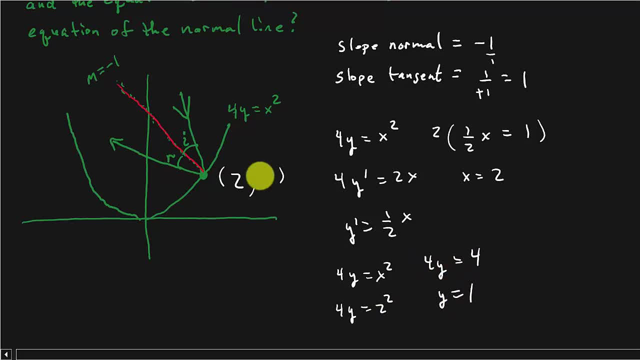 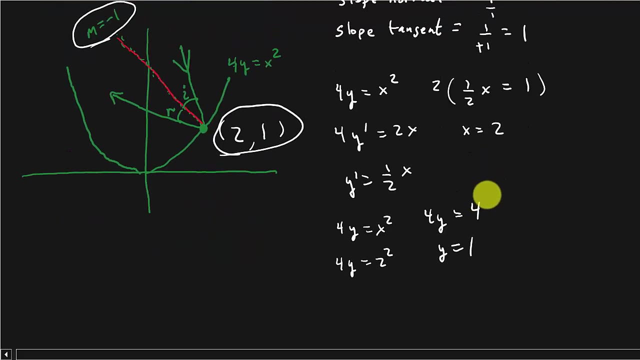 So 4y equals 4, y equals 1.. So that's the y coordinate of that point. Okay, And so can I find the equation of the normal line. Well, sure I can. I've got the slope, I've got my point. 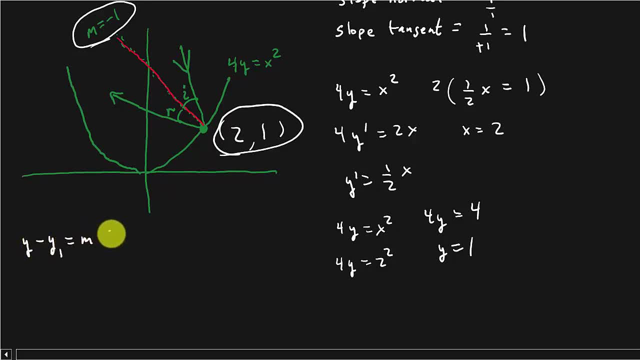 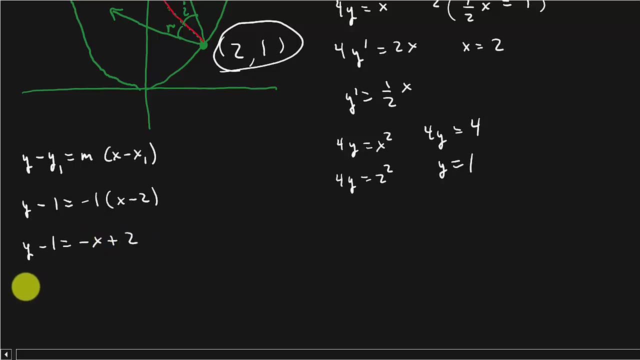 And so I'm going to use: y minus y equals m times x minus x, And so y minus 1 equals negative 1 times x minus 2.. And so this is going to be: y minus 1 is negative, x plus 2.. 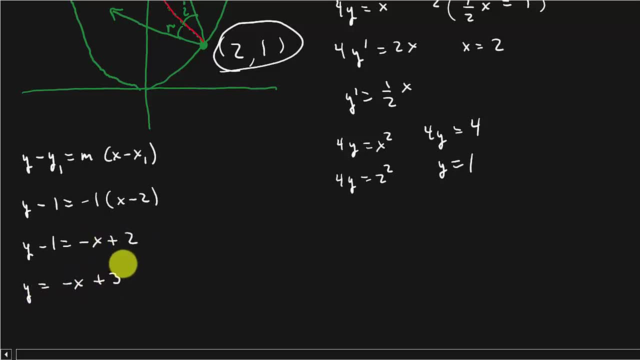 Okay, And so I'm going to use: y minus y equals negative x plus 3.. And that is the equation of your normal line. All right, So you know, for some reason this students make this difficult, and it's not. 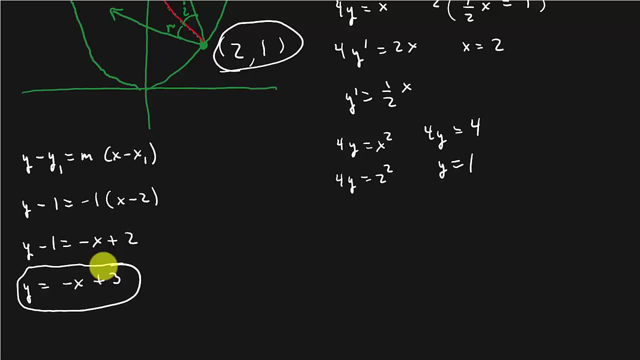 It seems like students. a lot of times they get the. if you ask them to find the equation of the tangent line, They typically get that one right, But it's. it's funny when you change that, change it from tangent and ask them to find.